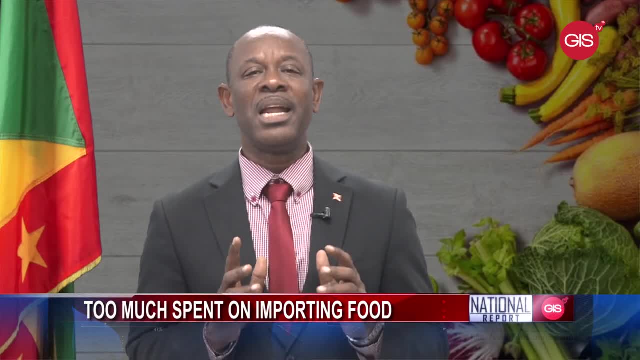 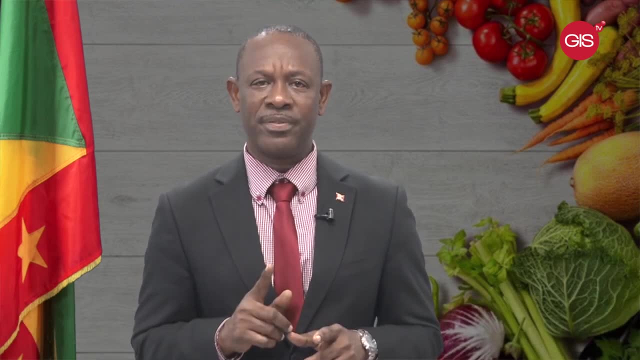 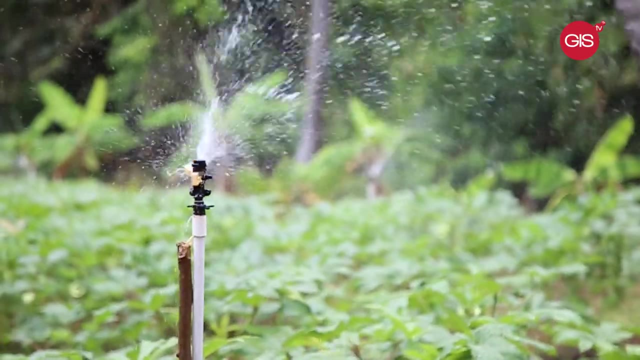 Minister for Agriculture, Forestries, Fisheries and Cooperatives, Senator Adrian Thomas, is calling on all citizens to band together to ensure our nation is food secure. Minister Thomas says the country is still staggering from the effects of the COVID-19 pandemic, the war between Russia and the Ukraine and other international tensions. 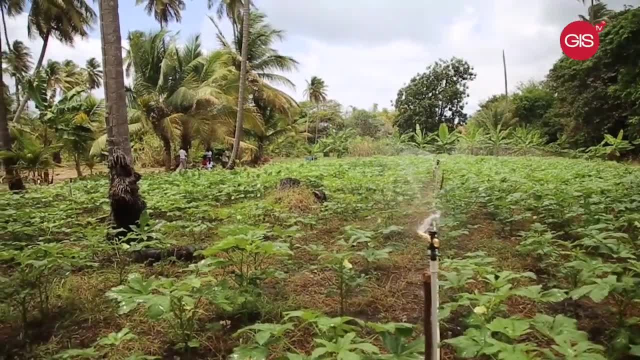 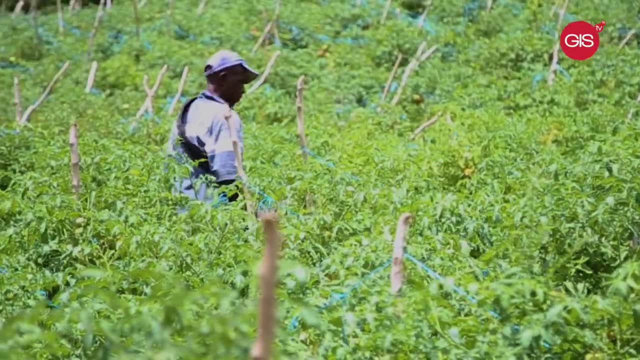 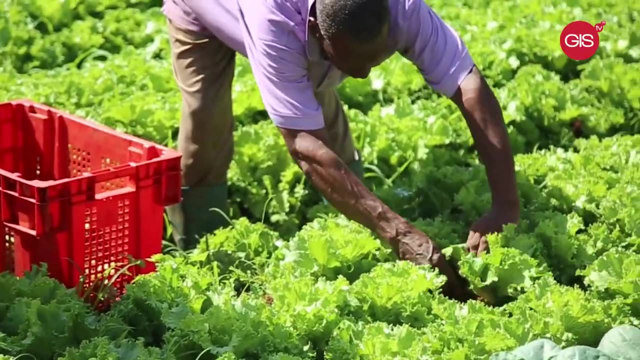 like global warming and the constant rise of food prices, which is adversely affecting food and nutrition security. Records show that the year immediately prior to the start of the COVID-19 pandemic, Grenada's food import bill amounted to EC 259 million dollars, whilst the country 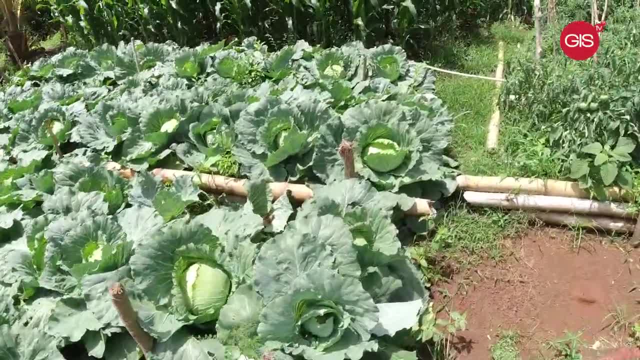 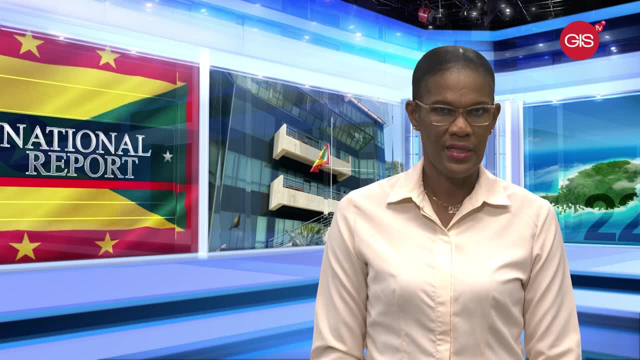 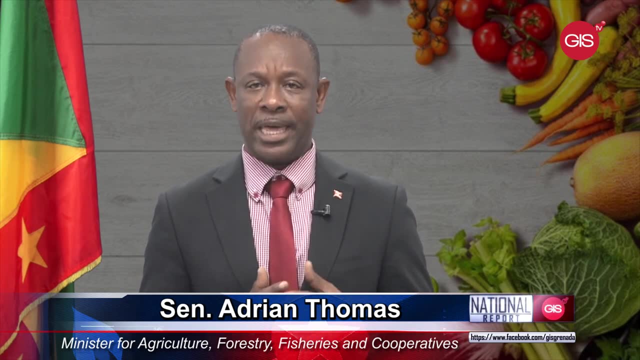 exported just over 79 million. During a message in observance of World Food Day, which was observed on Sunday, the Agriculture Minister says the high import bill is unacceptable and tackling this matter is high on government's agenda. There is a great imbalance between our imports and 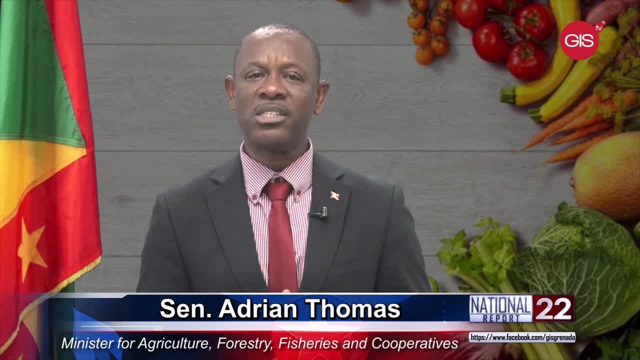 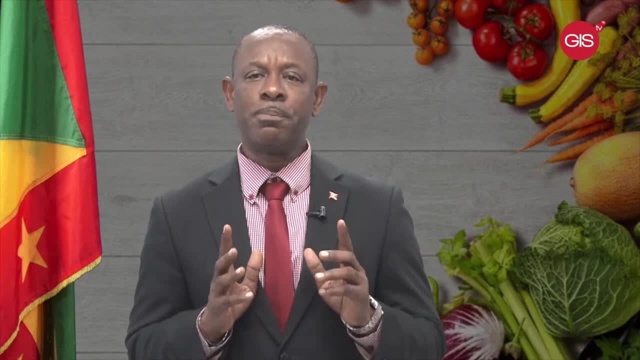 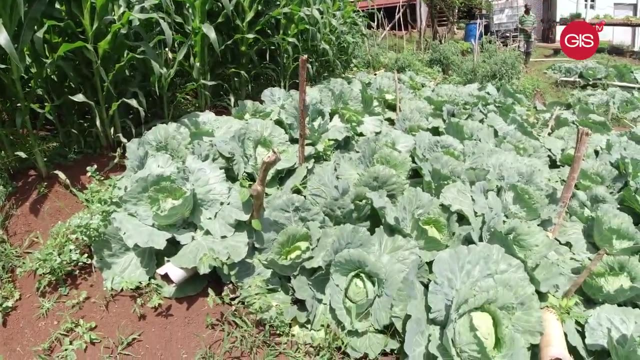 exports. This makes us highly susceptible to the impact of global activities on our food and nutrition security, and have been experiencing first-hand the negative impacts of the rising cost of food and fuel If only 10 percent of our imported produce is replaced by local grown foods. 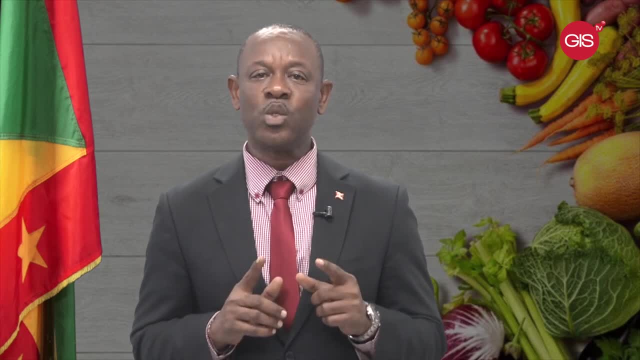 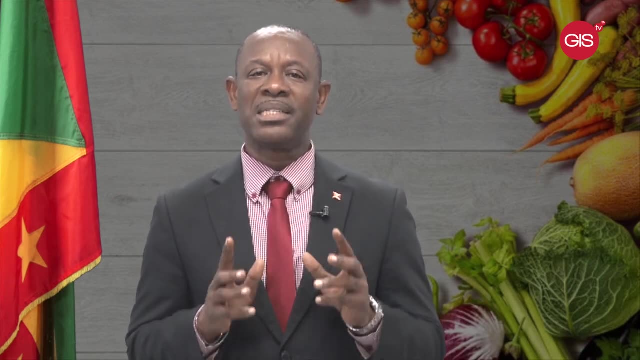 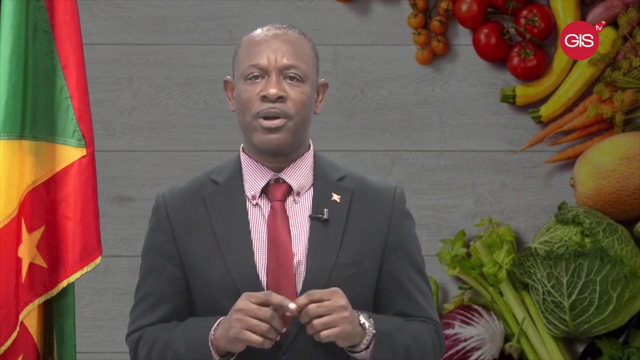 there would be an overall saving of at least 26 to 30 million dollars each year. This is one of the reasons our government has selected agriculture as one of the lead sector to contribute to the sustainable development, prosperity, health and wellness of our people. 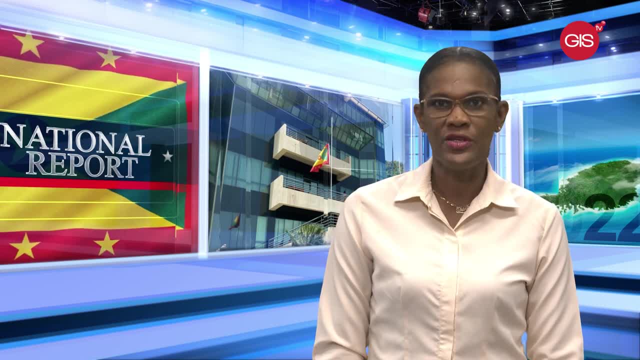 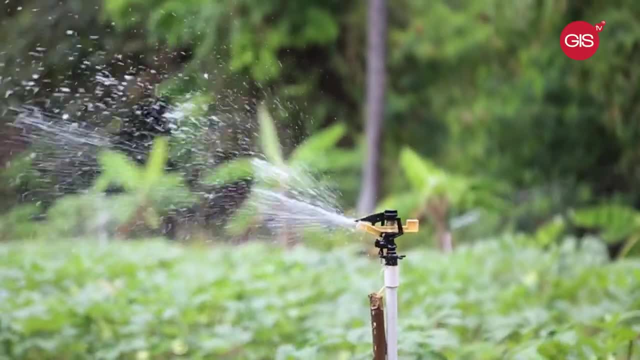 The theme for this year's observance of World Food Day is leaving no one behind, and so Senator Thomas is encouraging every citizen to get into the habit of growing their own food and supporting local growers and producers. He says government is providing the leadership in promoting and. 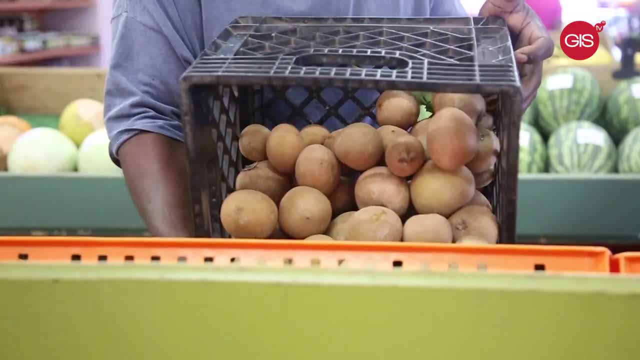 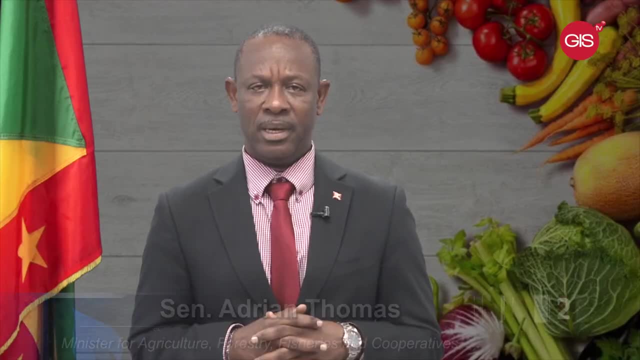 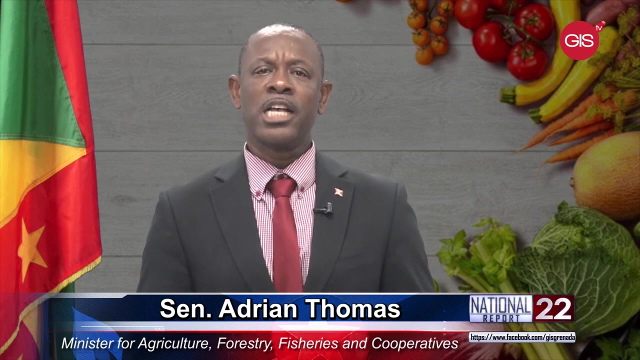 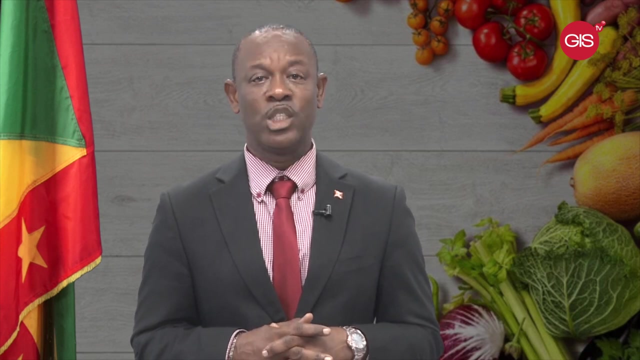 developing sustainable agricultural policies, plans and programs that would boost food and nutrition security, as well as attract the younger generation to the agriculture industry. The Ministry of Agriculture and Lands, Forestry, Fisheries and Cooperatives has prioritized the national food and nutrition policies for review and implementation in 2023.. This policy aims to